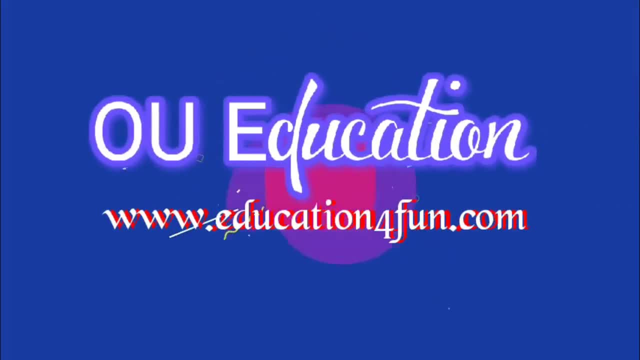 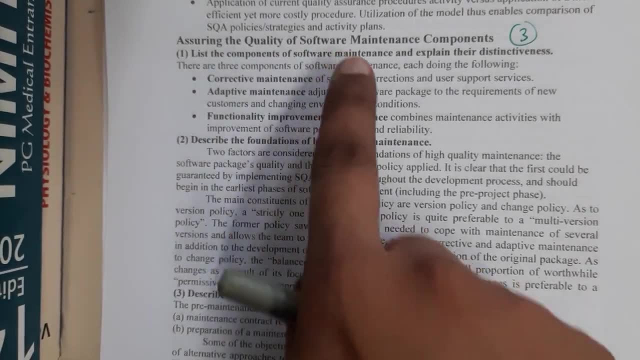 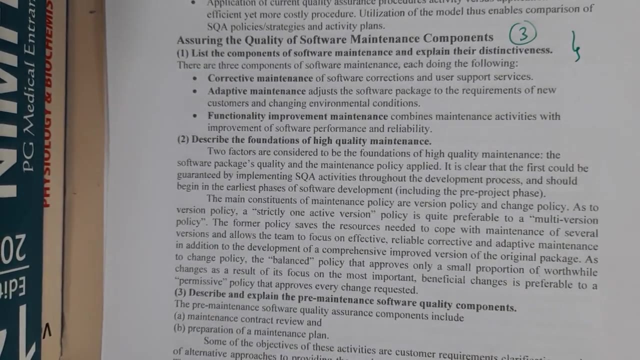 Hello, guys, you're back with our next lecture. In this lecture, let us go through the concept of assuring the quality of software maintenance components. Okay, guys, I tried to understand from the notes which I have shared, but it's not that much good for this concept, guys. So that is. 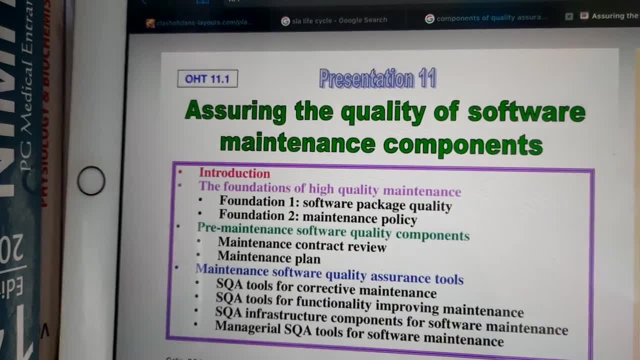 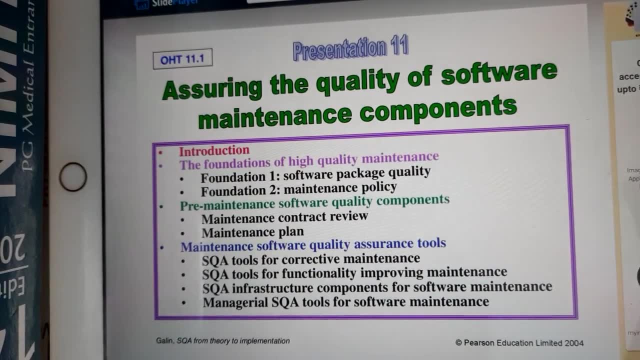 the reason why I searched for a PPT and I found the PPT of the textbook itself. So, basically, the textbook PPTs are available. Okay, yes, So I'll be using this PPT to explain guys, I'll be downloading it and I'll be sharing in the groups also, Don't worry. Okay, Yes. So once the videos are live in. 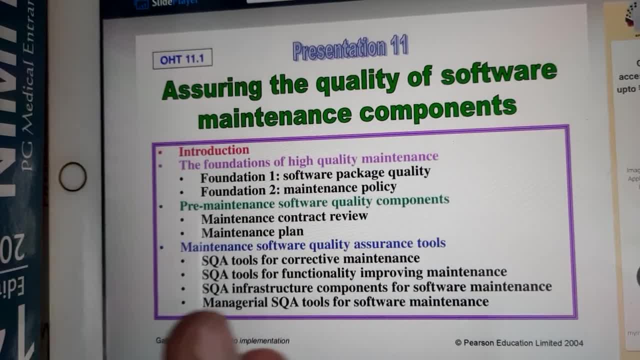 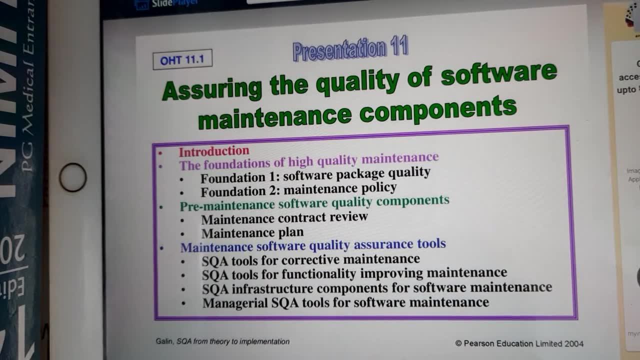 around one to two hours. we'll be getting this PDFs also, Don't worry. Okay, Yes, So basically assuring the quality of software maintenance components. So basically assume that you created a software. Okay, So once you made the software, will you update it or will you maintain it, guys? 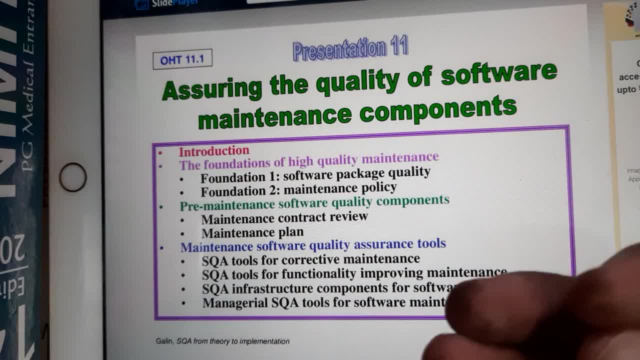 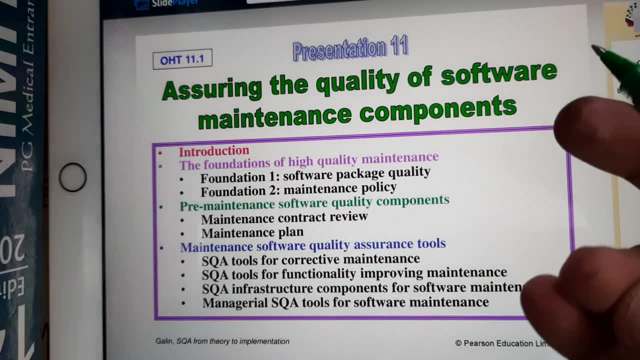 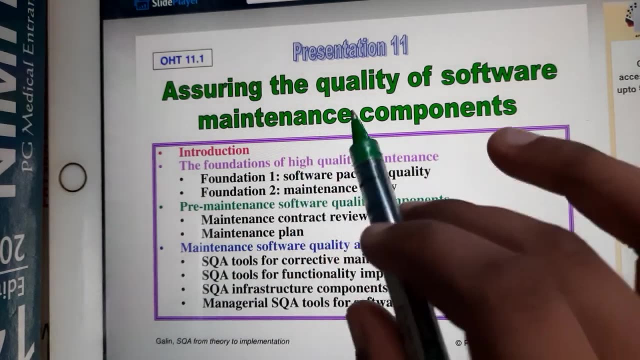 So basically, few softwares or few games will not have this updates and maintenance frequently, Right, Yes, So that is the reason why always the maintenance and the updates are pretty required for a software, because any kind of bug fixes and all those issues will be resolved in this maintenance and all these phases. guys, Okay, Yes, So firstly, 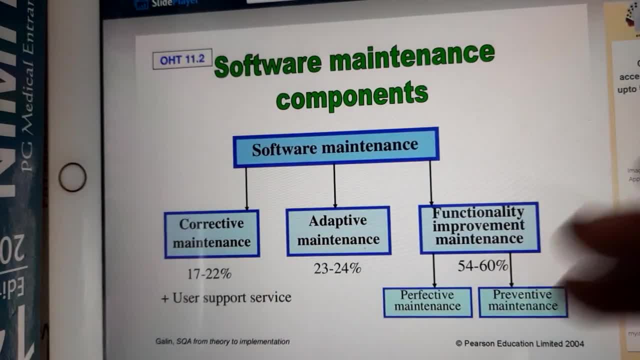 let us go through the components. So what are they having? So what do we exactly maintain? So, basically, software maintenance is divided into three different parts, You can say. So the first is a corrective maintenance. Okay, guys, we'll be going through the small. 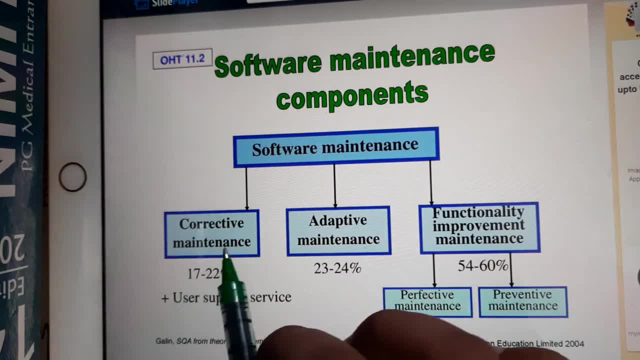 small, one line definitions for these three components, Don't worry. Corrective maintenance, which is 17 to 20.. 22% of the whole software maintenance. Similarly, adoptive maintenance, which is 22 to 24% of the whole software maintenance. Similarly, functionality improvement maintenance, which includes two that. 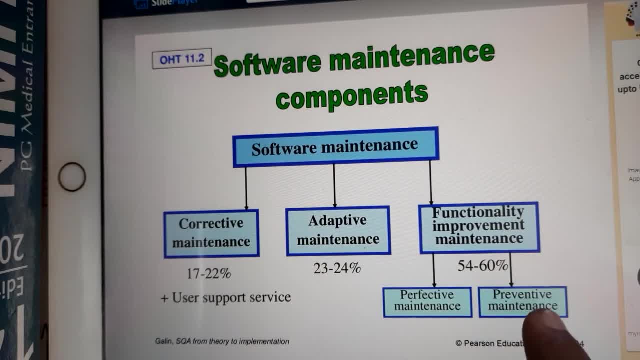 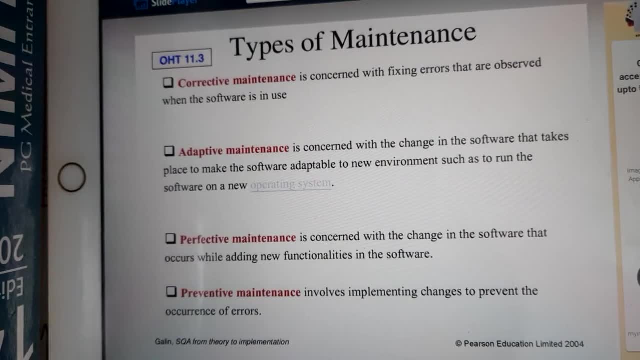 is a nothing but perfective and preventive maintenance. Okay, Yes, So these are all the components. you can say, guys, Okay, Yes, So let us continue with their types and let us go through some small, small definitions. You can say: Okay, Yes, So the first one is a nothing but. 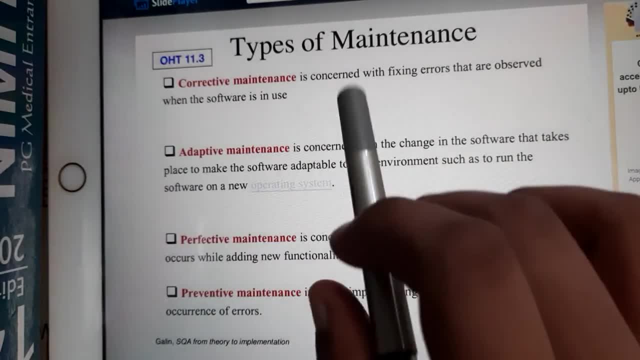 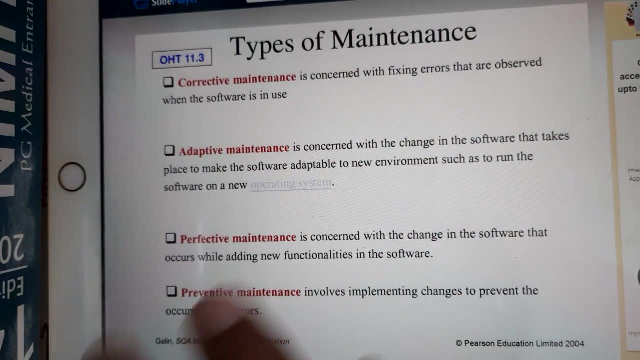 corrective maintenance, right? Yes, So corrective maintenance is nothing but is concerned with fixing errors that are observed when using the application. So assume that you are using the application and you found some bugs or issues, So those comes under the corrective maintenance. Okay? So, basically, if you understand, so let me give you an example here. 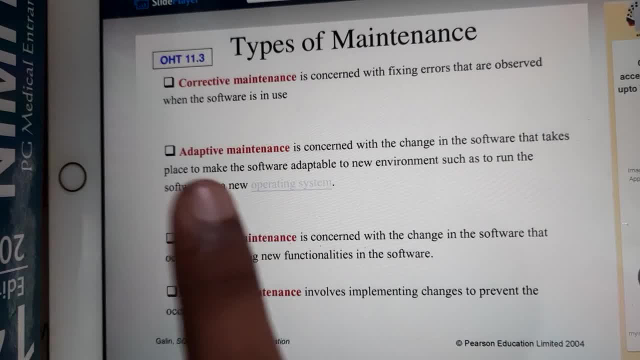 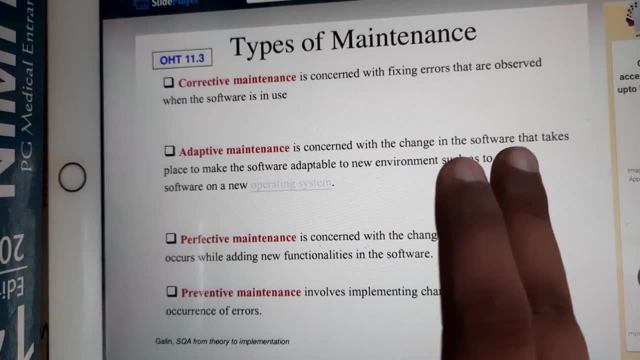 itself. So whenever you are using guys, this is a slide from the slide player directly. Okay, Yes, Okay. So basically, whenever you assume so when you press on the right side it should go to next slide, right, It's going. But when you press on the left side, 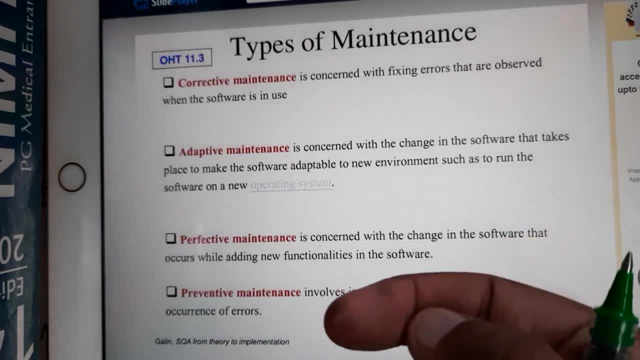 it should go to next slide. So when you press on the right side it should go to next slide, It should go to previous slide, but here it is going to next slide. So this is a small bug. you can say or issue. you can say: Okay, Yes, I don't know exactly how this slider is built Like. 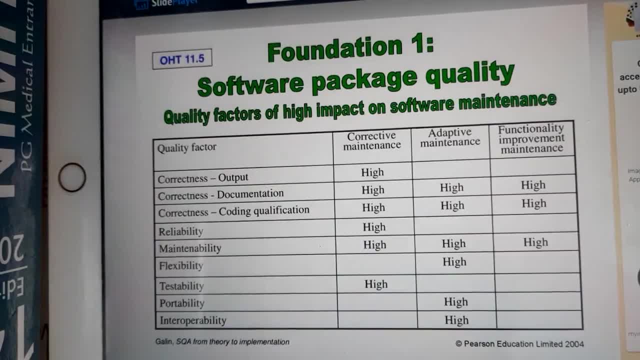 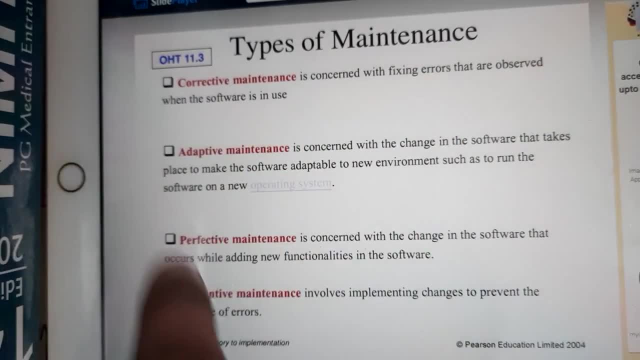 anywhere you press, it will be going to the next slide only. Okay, Yes, So that that kind of things which a user can find. So those comes under the corrective maintenance. So these will be corrected in the corrective maintenance. Similarly, adoptive maintenance: Okay, So is. 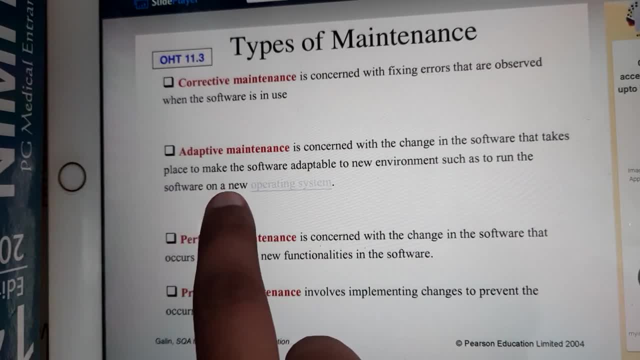 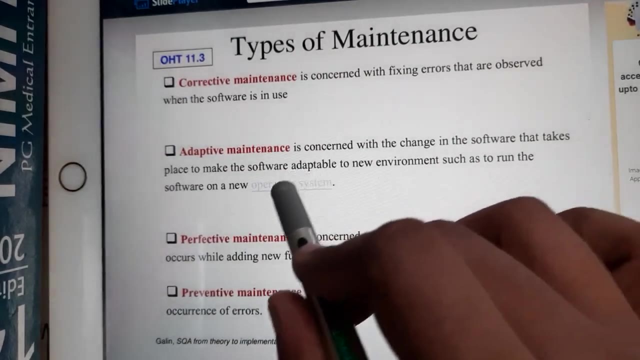 concerned with the change in the software that takes place to make the software adoptable to new environments, such as a running software, new operating system. Okay, So assume I hope everyone knows the news that windows 11 is going to come pretty soon, right? Yes, So assume that. 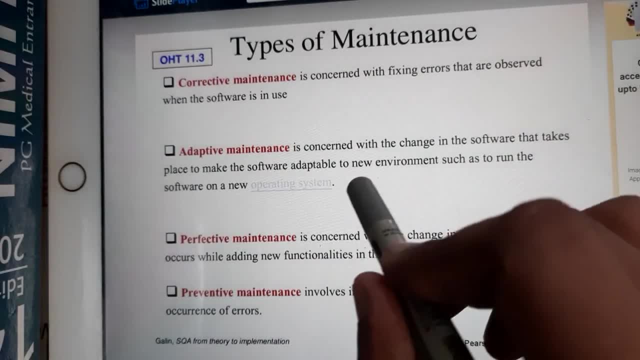 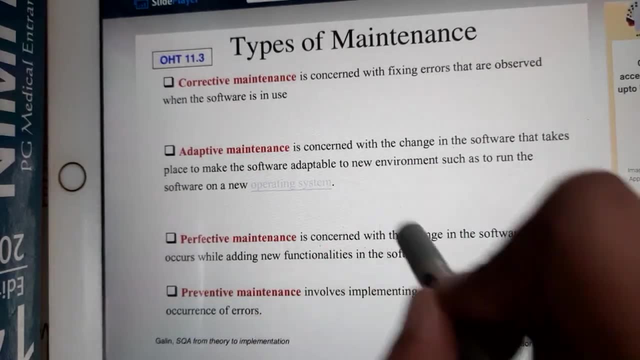 there is a software which I developed in windows 10.. Okay, So now my goal is to migrate it or make it possible to work in windows 11 also. So that is my goal. So, in this way, if you are adopting to some particular new operating system or a new environment, so assume that I built an. 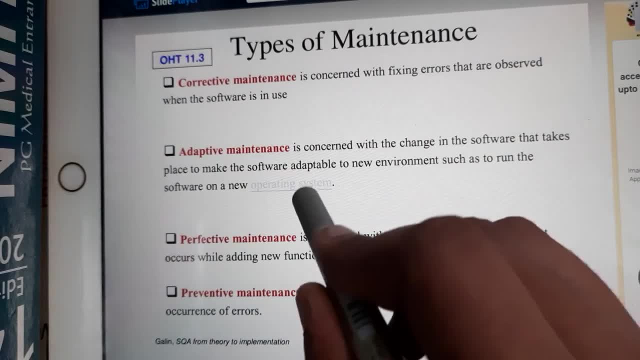 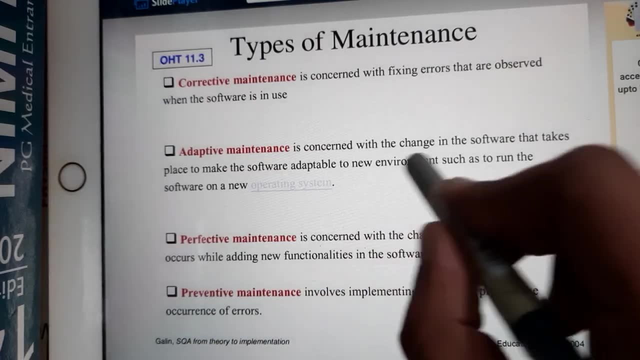 application for windows. Now I want to build one more application for Linux, but I don't. I don't want to change anything in this, So I need to convert this. So these maintenance, like making it possible to run in another OS, is nothing but your adoptive maintenance. guys Got it. 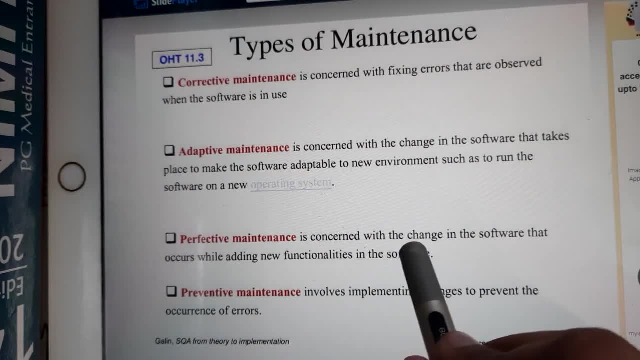 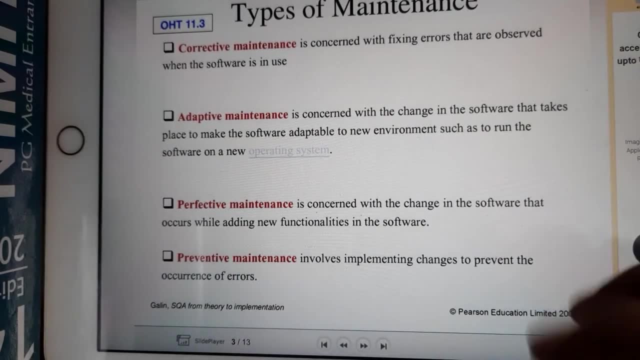 Yes, Similarly perfective maintenance. So is concerned with the change in the software that occurs while adding a new functionality in the software. Okay, So assume that previously your application did not have download option guys. Okay So this has download option, but assume in. 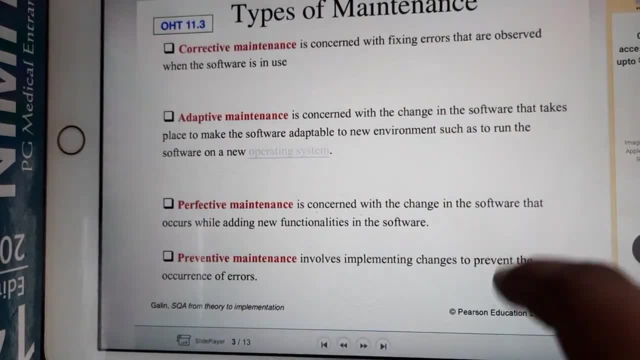 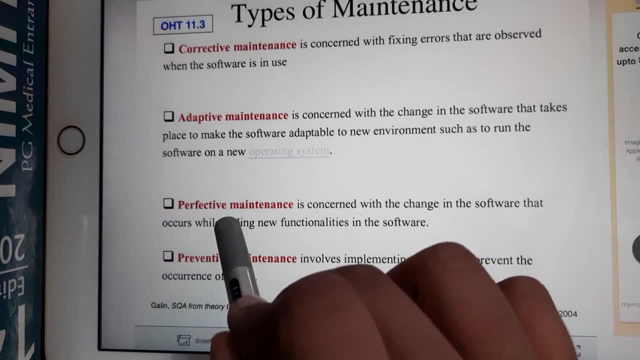 that way. Okay, So in that situation you will be add, you added that download option, So you are adding some new functionalities right In a maintenance break. So that is called as a perfective maintenance, guys, Okay. Similarly, the last type is a nothing but preventive maintenance. 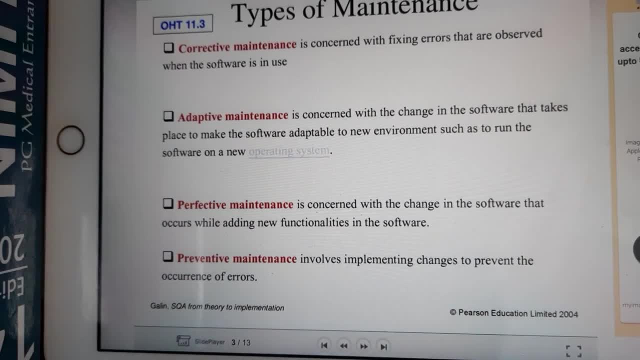 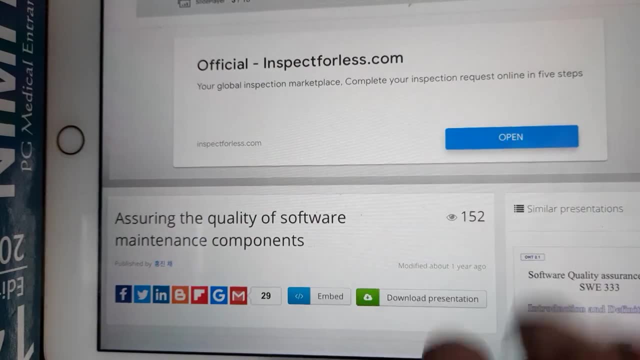 Okay, So it involves implementing changes to prevent the occurrence of error. So assume that the download button is not working. Okay, So in that situation you held a maintenance break for one or two hours and you repaired that maintenance button. So that concept is nothing but preventive. 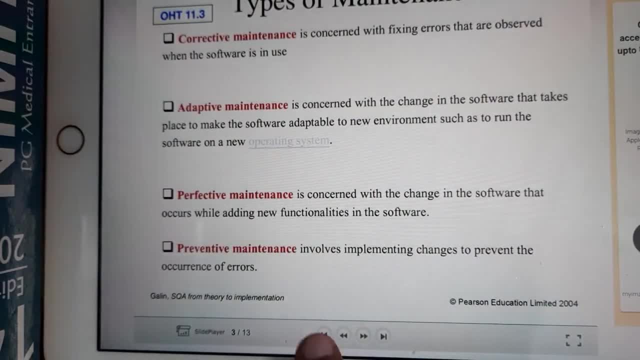 maintenance, Got it? So these are the four different types of maintenance and you can draw this diagram, guys, to showcase them. Okay, Yes, So I hope everyone got a clear idea about this. maintenance for types, right? Yes, Okay, So I hope everyone got a clear idea. So what are? 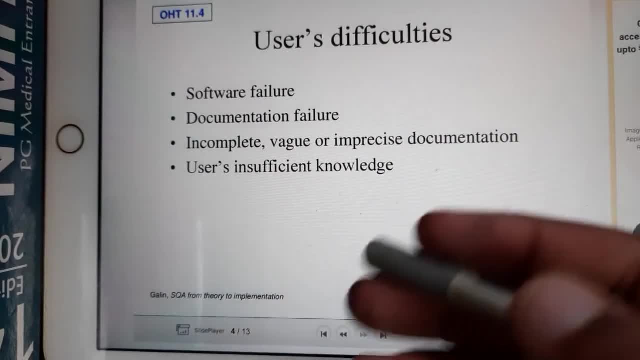 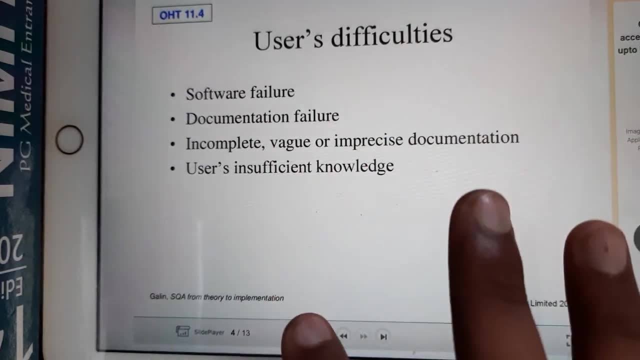 the difficulties which a user can face, guys. Okay, So the differences are the difficulties which a user can face is some software failures. So basically, when you are using the application, suddenly the application will close or it will force stop. So that comes under the software. 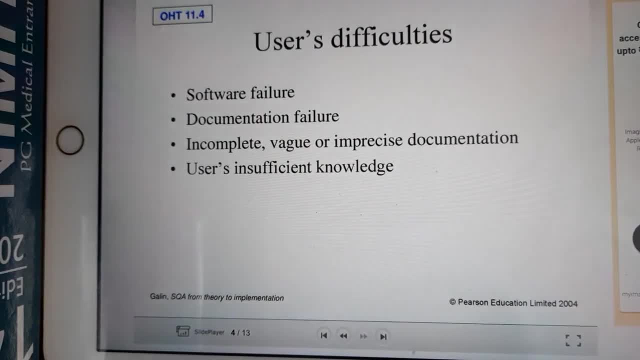 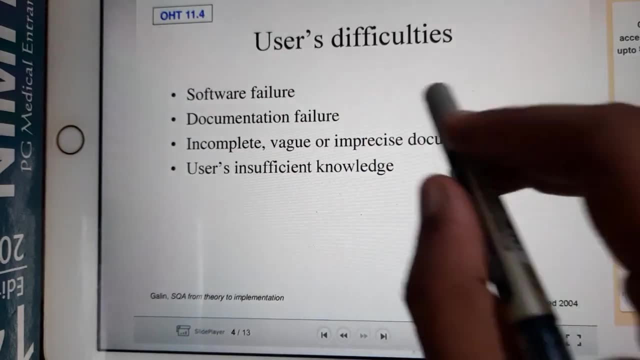 failure and it's similarly documentation failure or documentation is incomplete. So assume that you have a document for the users to read, like user manual, which most of the applications will give So that manual you created, but it's not opening in the user's end. They cannot read it properly. 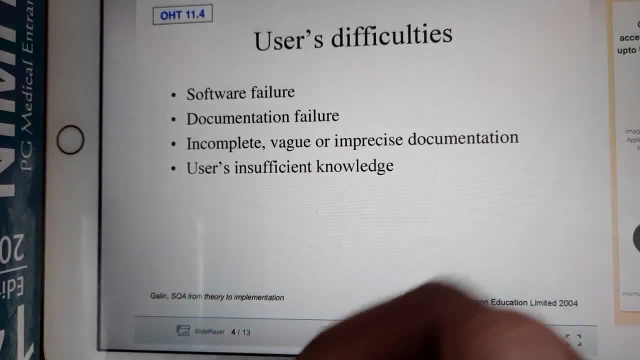 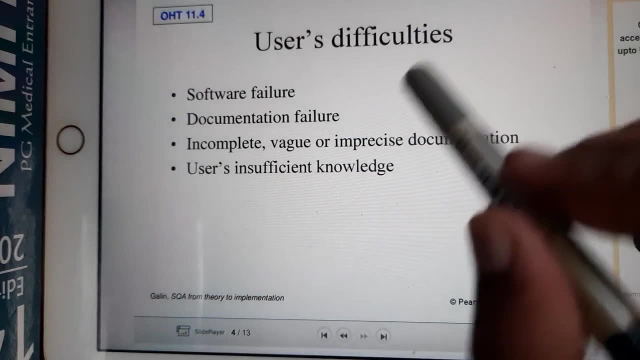 There are some line breaks which are missing. Few lines are missing. So in that way, if they are missing, so the document failure will comes under that. Similarly, incomplete documentation, So this also comes under that. and user insufficient knowledge, So assume that in your documentation. 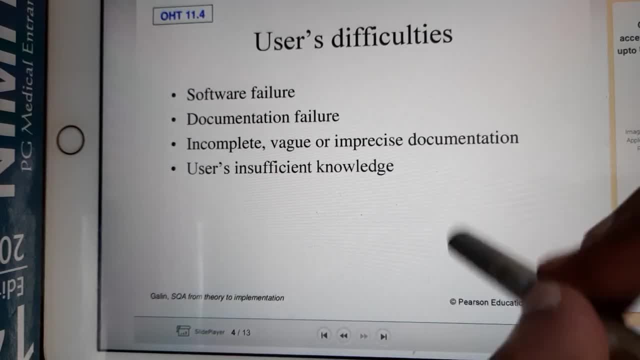 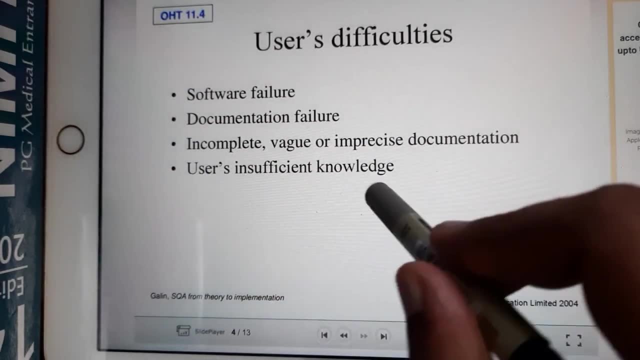 you mentioned your code, how your code works, how your things will work, And you are giving this to the end user. So, basically, the end user requirement is not to learn the coding or the concept behind your program, right, Yes, So in this situation it is a waste of his time to understand those things. 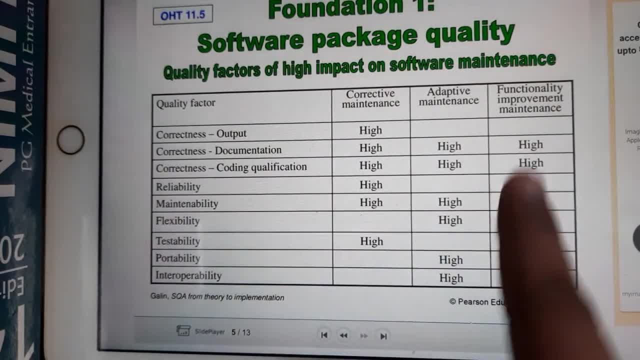 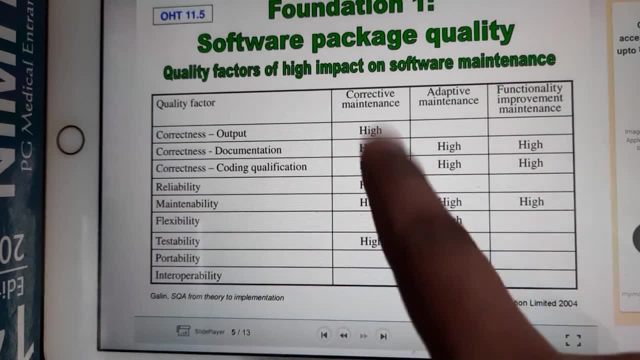 So that will also be an issue, right? Yes, Okay. Similarly, these are some table. This is a table guys, which shows the importance. So, basically, correctness on the output will comes under which maintenance? So it comes under corrective maintenance, because you are checking the output. 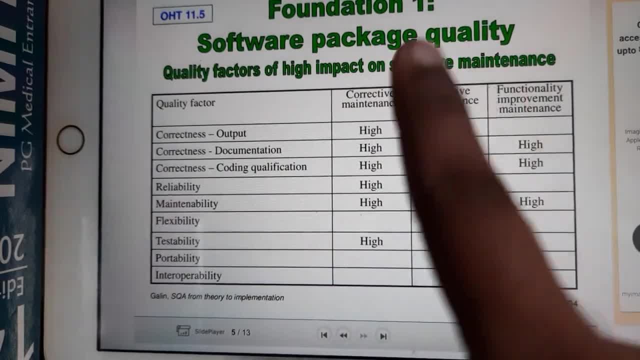 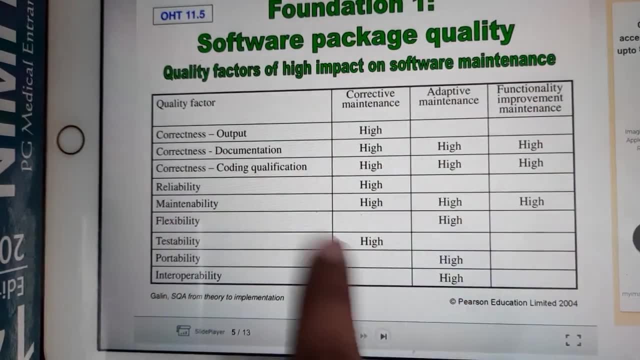 So in this way this table is mentioned. I guess please go through the table and please remember it, guys, because maintenance, the software maintenance question could be expected, because this is an interesting topic, right? So the evaluator might ask in this topic. So please make sure that you are going through the.